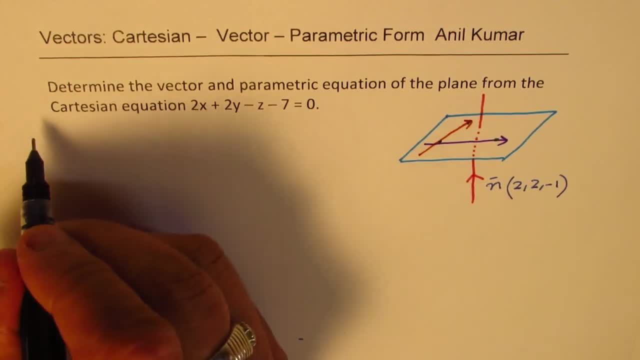 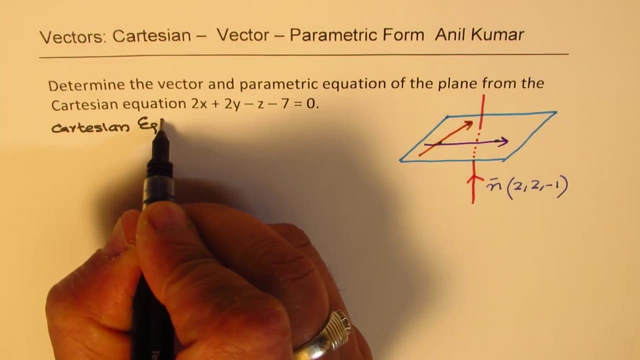 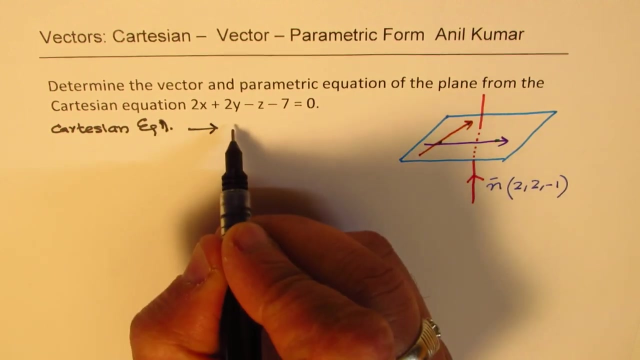 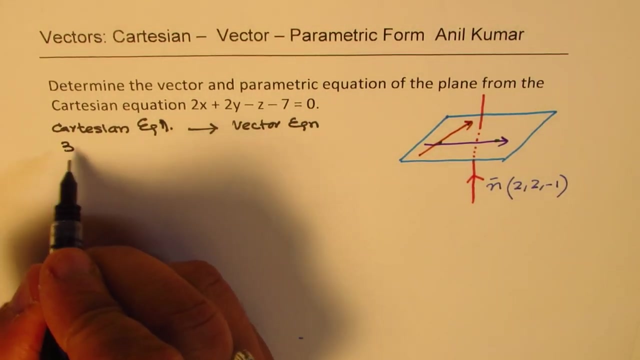 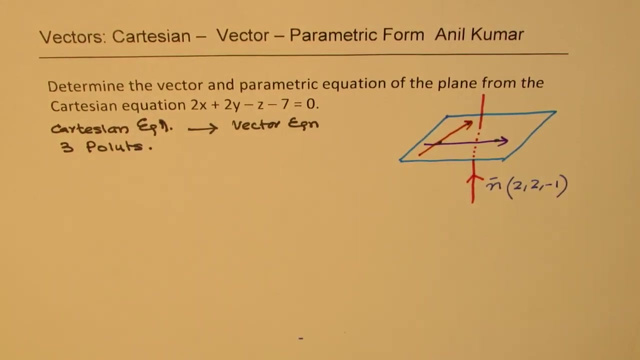 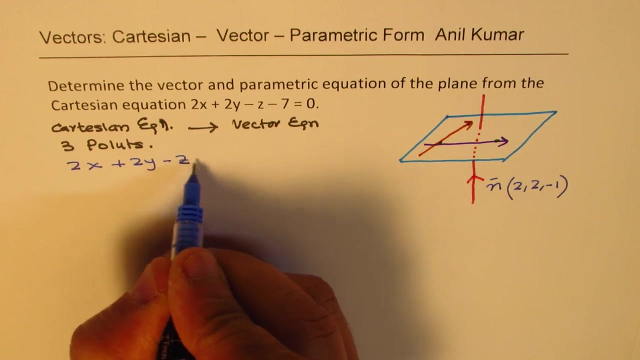 got the concept. So the first step to write a Cartesian equation, let's write it, and from there to get vector equation. what should we do? We should find three points correct. So, in the given form, what are we given? We are given an equation which is 2x plus 2y, minus z, minus 7 equals to 0. 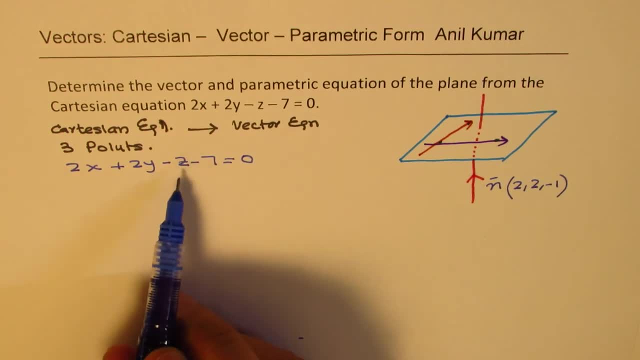 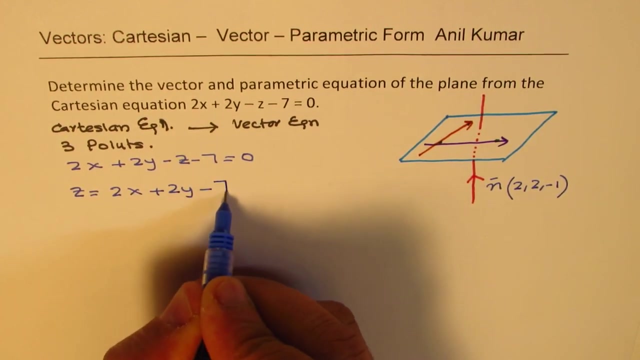 Now plane has infinite points. We should make our work simpler by isolating the simplest of these parameters. So z. if I take it on the other side, I can write z as equal to 2x plus 2y minus 7,. 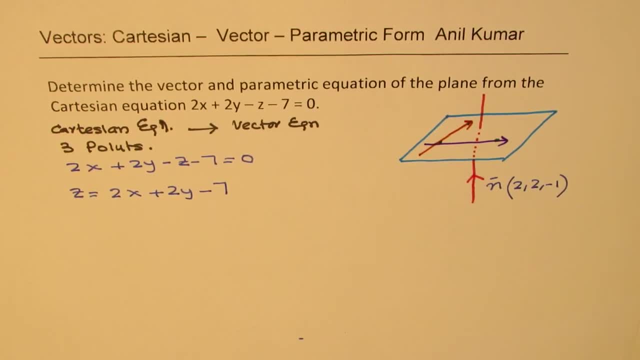 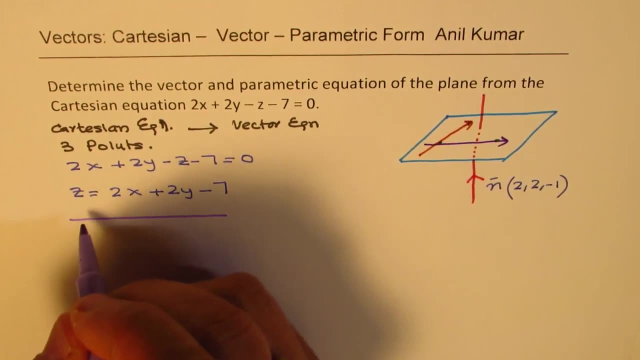 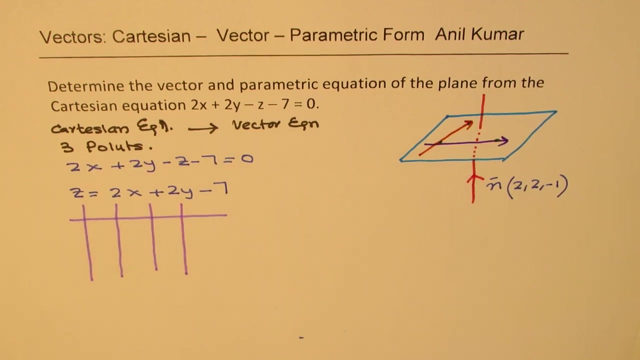 correct. Now for different values of x. we can find the value of z, right. So we will just make a table here And find three points Giving values to x and y. right, We will calculate what z is. 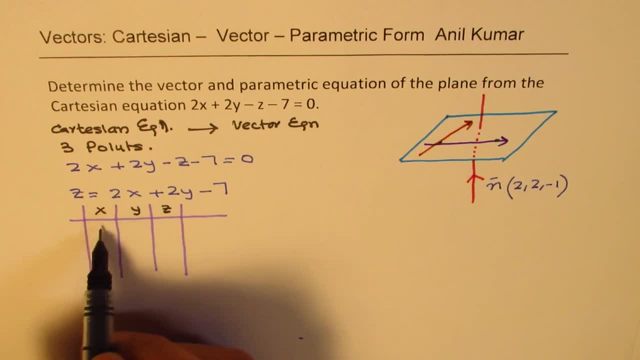 So here, if I write a value, let us say 0 for x, right, And let us say 1 for y, In that case z will be equals to: this is 0 and that is 1.. So it is minus of 5.. 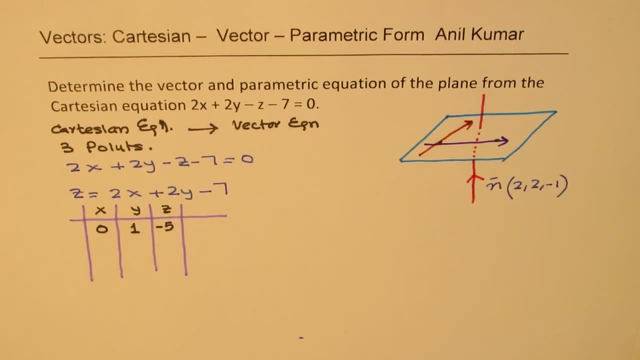 Correct. So just substitute the values here and get your z value, So that becomes first point for us. Now we could do something like this: I could have placed 1 for x, 0 for y, So 1 means 2 here. 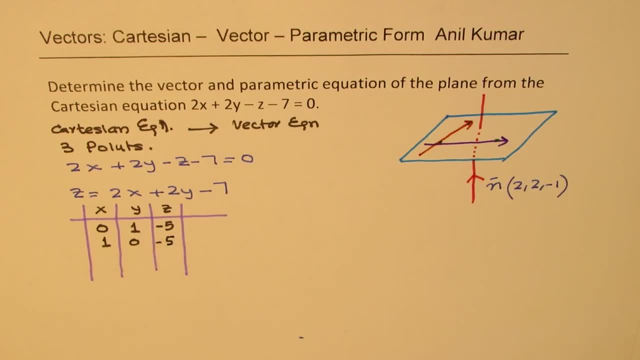 and 2 minus 7 is again minus 5.. So I got two points correct. We can also place both of them as 0, right? So we could take 0, 0 and minus 7.. So that gives you the third point. 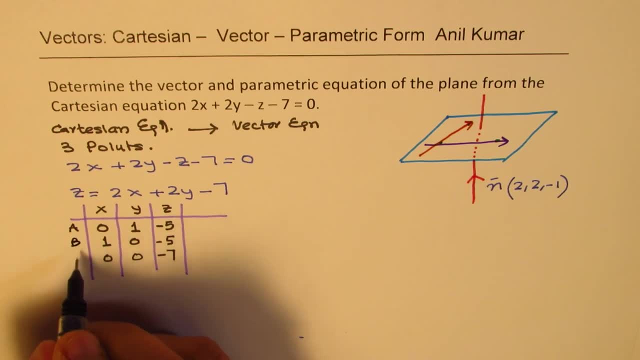 Let us call these points as a, b and c. So now we have three points. With the help of these three points, we can find two directions. right, We can find two directions, And from those directions we can get the vector equation. Does it make sense to you? I think it does right. 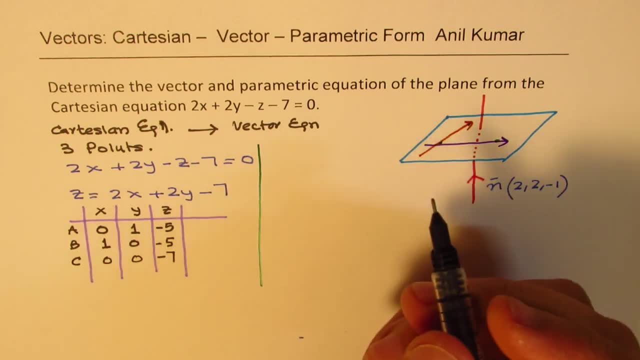 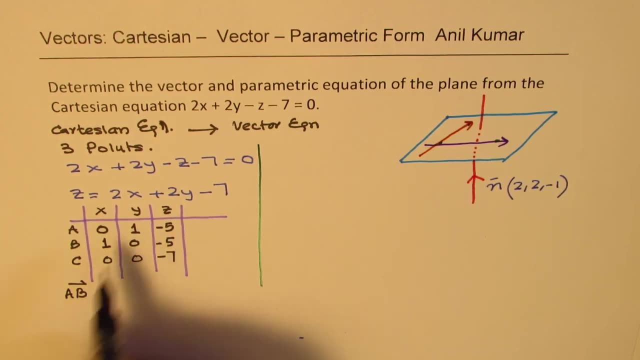 So let us find the two directions. So let us first find what is our direction a- b. We can do it here also, right? So what is the direction a to b? So a to b, these are my points, right? So it will be b minus a. So let us write like this: So: 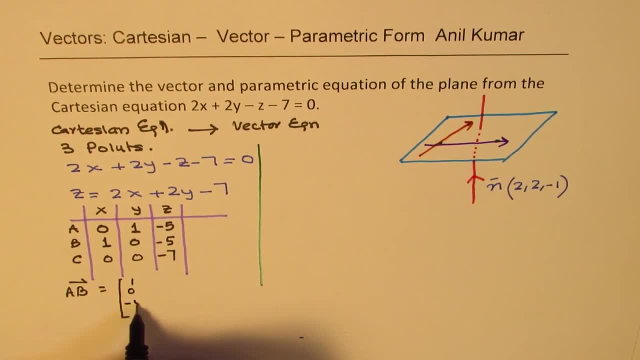 b is 1, 0, minus 5.. And from there we will take coordinates of a, which is 0, 1, minus 5.. So what do you get? a to b? a to b is 1, 1 and 0. So we get a to b. Similarly. 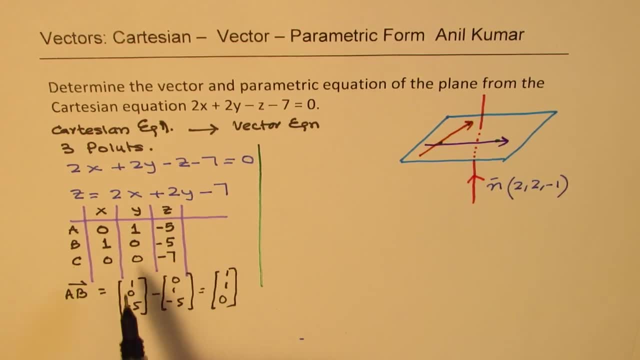 we can find what b to c is right, So let us find b to c, So b to c will be equal to. we can do from here 0, minus 1, right? So we could also write this in this form So: 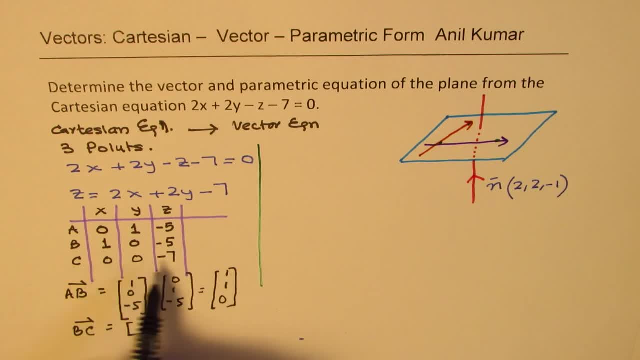 these are different forms. since I have lesser space here, So I will just go horizontal this time. So b to c is c minus b, right? So this minus this gives me minus 1.. That gives me 0.. And this gives me minus 1.. So this minus this gives me minus 1.. That gives me 0. And this gives. 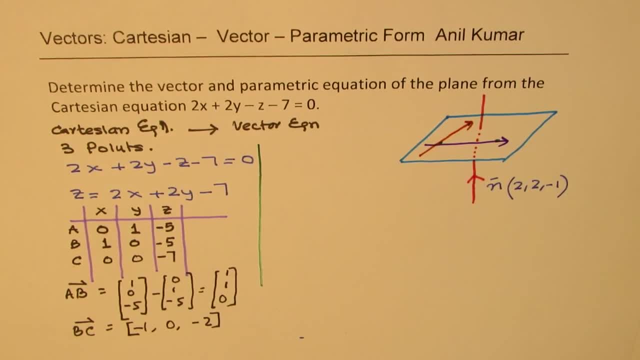 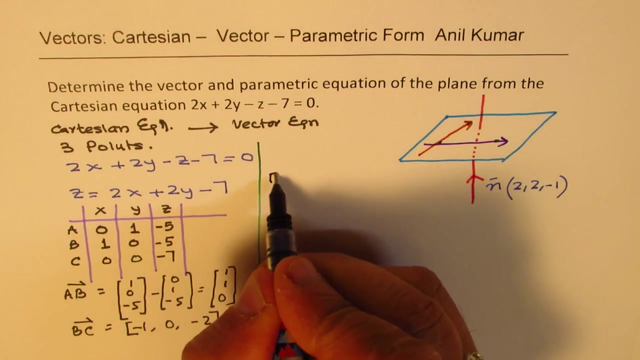 me minus 2.. So I get two directions. Perfect, I could have written this as c to b also. Now, with these two directions I am in a position to write down the vector equation. So the vector equation for this particular plane will be: we can use one of our points, which is 0, 1, minus 5,. 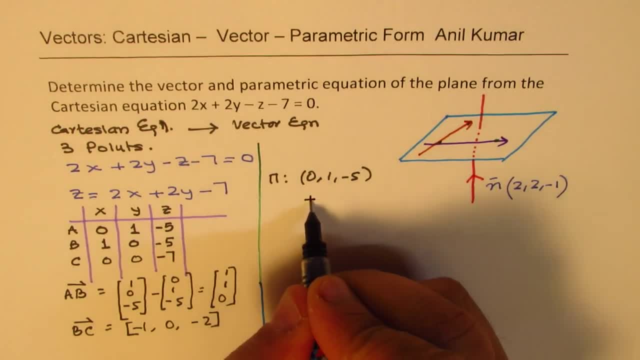 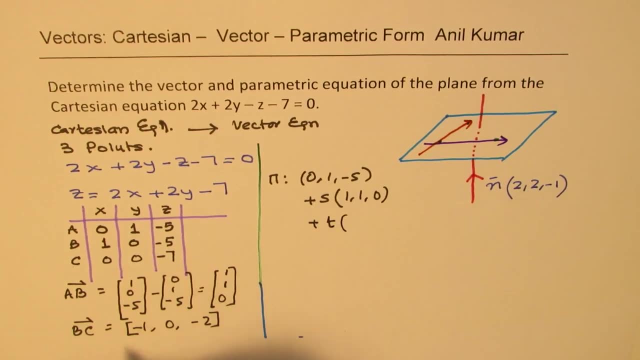 correct And we will use a parameter. So we will say plus s times one of the directions, which is 1,, 1, and 0, plus t times the other direction, which I could also write as 1,, 0,, 2.. It is very important to understand. both are same things. 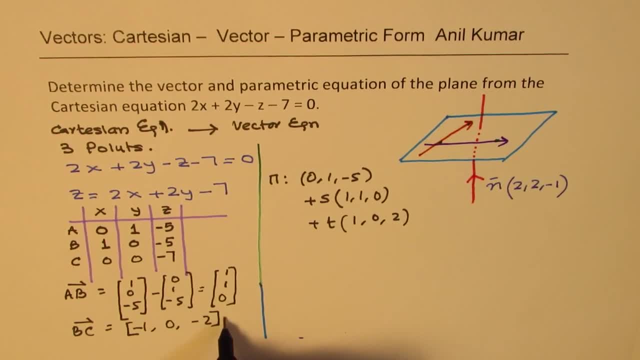 okay, We are just taking a parameter right, Which is actually same as you can take minus common right, 1,, 0,, 2.. I could have written c, b right, So in a way, as the direction is concerned, it is kind of same right. So in my vector equation, 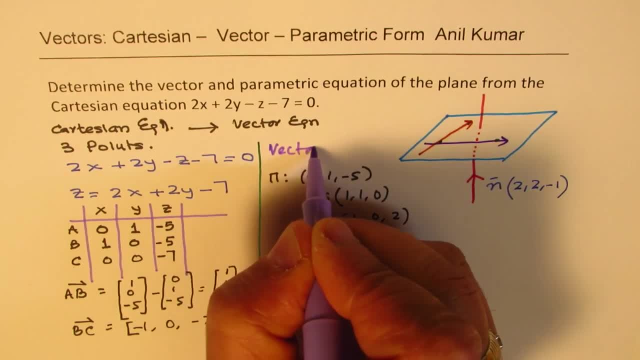 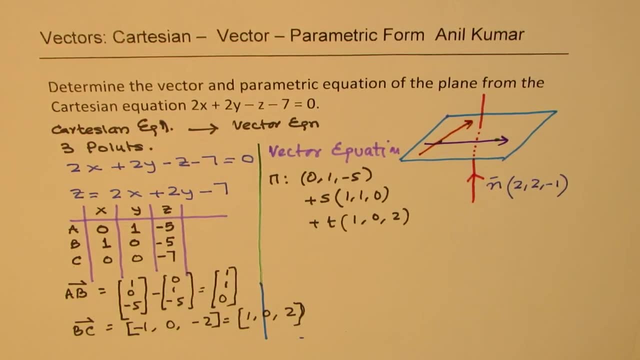 I could write that as my answer. So that becomes my vector equation Clear. Now, how do I get my parametric equation? Well, that is simple: We will write parametric equation from a vector equation. So from here you can clearly understand that these equations are not unique. 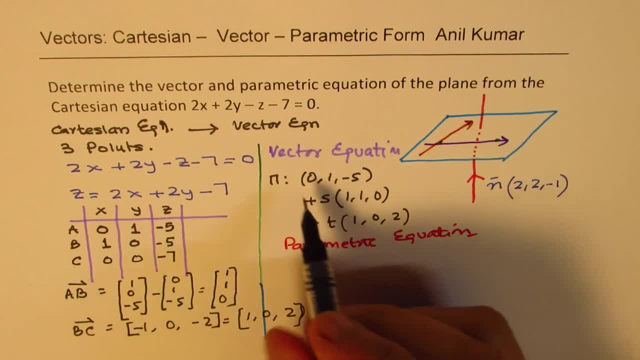 but scalar equation is absolutely unique, right? So from our vector equation we can say: x is equal to, so this is 0,, right? So we could write this as s plus t. y is equal to 1, plus s, right. 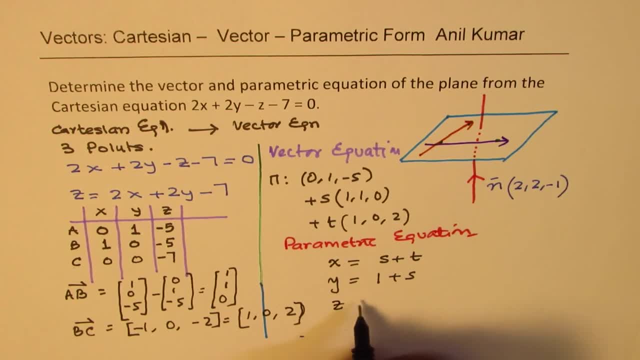 0 parameter, That would be 0. And z is equal to minus 5.. That is 0. And this is plus 2t. So that becomes your parametric equation. Doesn't make sense to you, right? So that is how you. 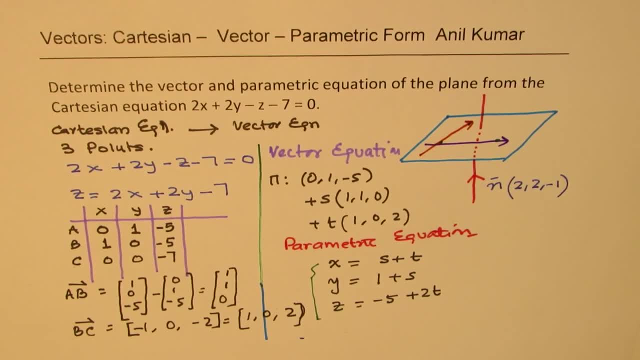 could actually get vector and parametric equation from the given Cartesian equation right, So you could find any set of points, no restrictions at all, Perfect. You could have written a, b. You could have written as we later did. we wrote: 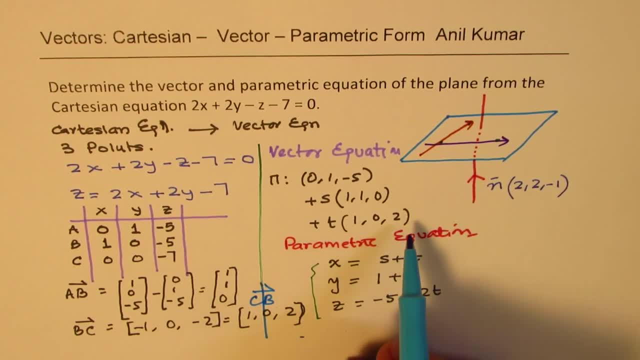 this as c, b, right And use that direction in our example. We normally avoid the negative signs in the direction, especially for the first one. okay, So I hope that makes sense. Feel free to write your comment, share your views and, if you like, and subscribe to my 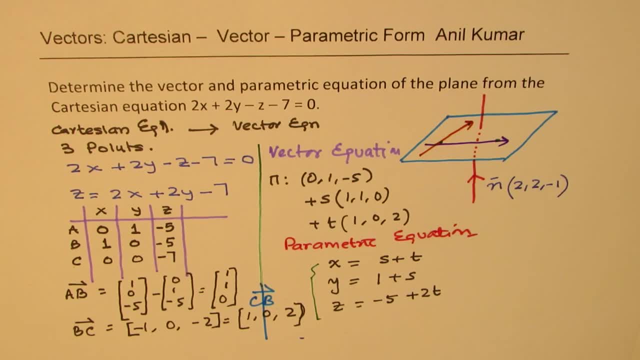 videos. that'd be great. Thanks for watching and all the best.